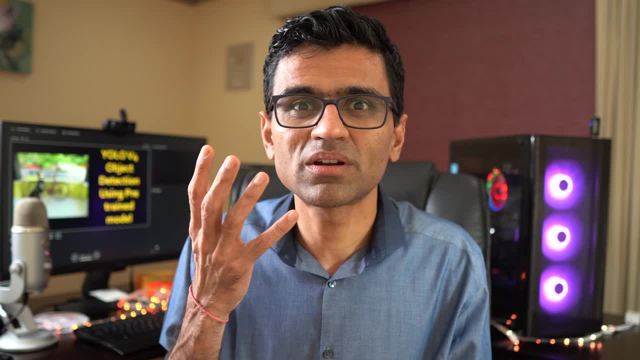 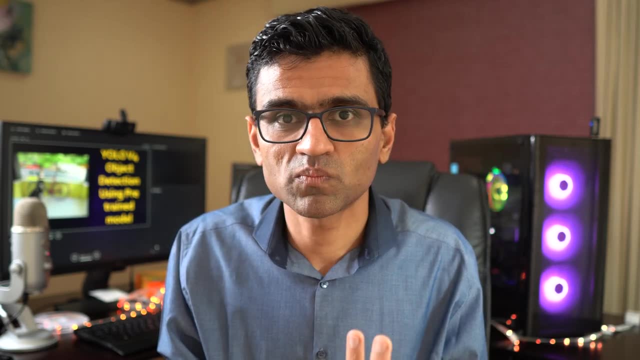 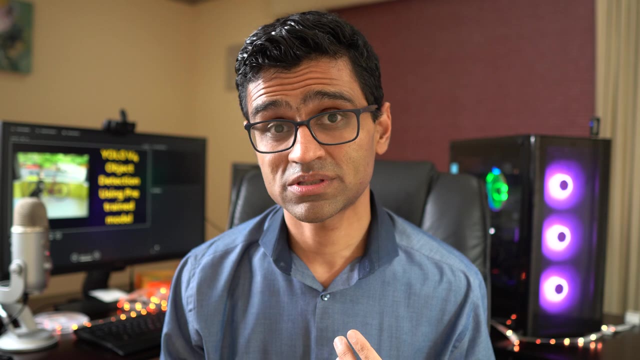 profile is such that it's see, in the end it's all economy, supply and demand. there is enough supply of data analyst in us, so why would they? you know they're like american citizens- green card holders- why would they go into hassle of filing an h1? because they have to respond to government that. 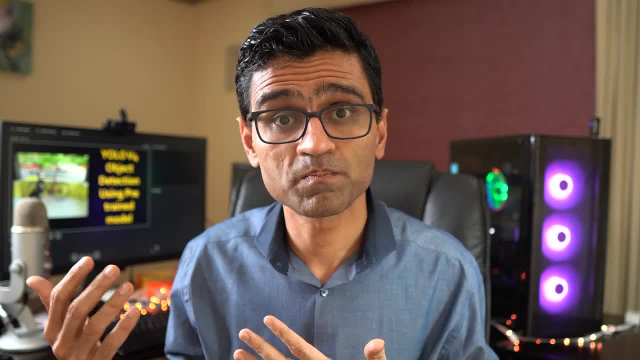 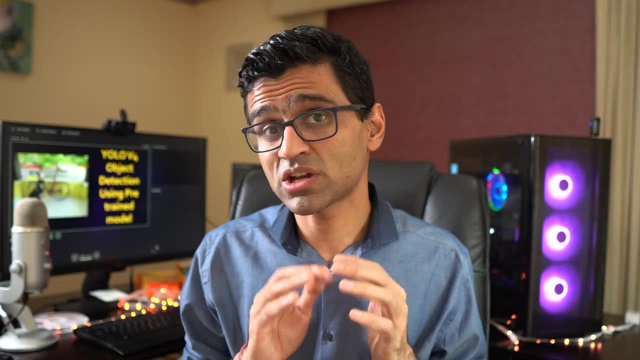 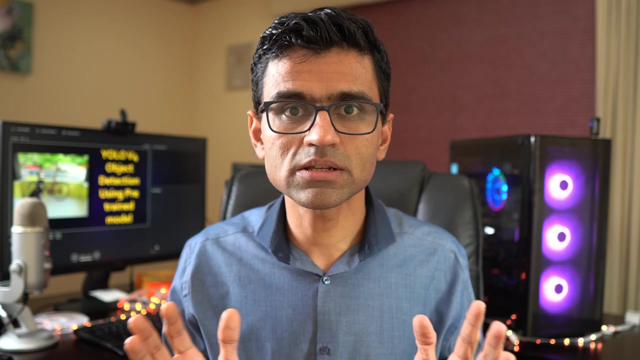 they are not finding a good, talented employee locally, hence they're filing h1b. they would not go through that trouble, so they make it an hr policy that for data analyst profile, we are not doing any h1b. so the short answer is: if you are coming, thinking of coming to us to become data analyst masters? 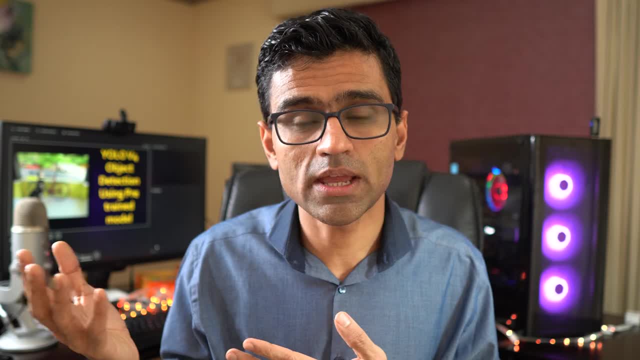 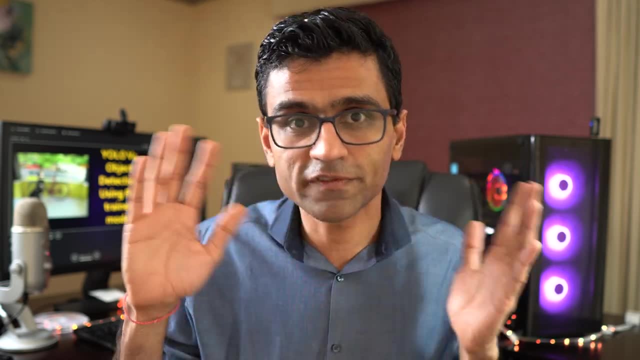 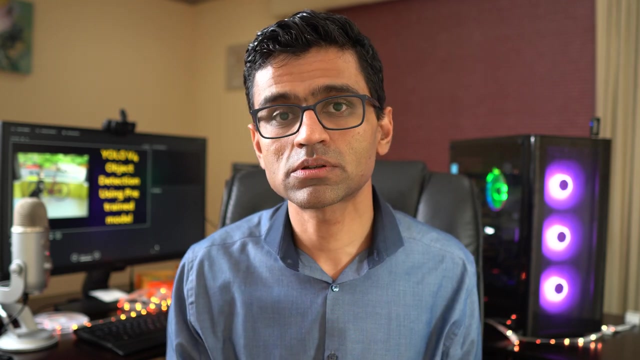 and work here on h1b- not a good idea. now, you might get lucky. i'm not saying, see, you might get lucky. maybe one person case people even get h1b, fine, but you have to be ready, uh, to take that much risk. so evaluate the options in your home country. there are enough jobs and so many career options, so many. 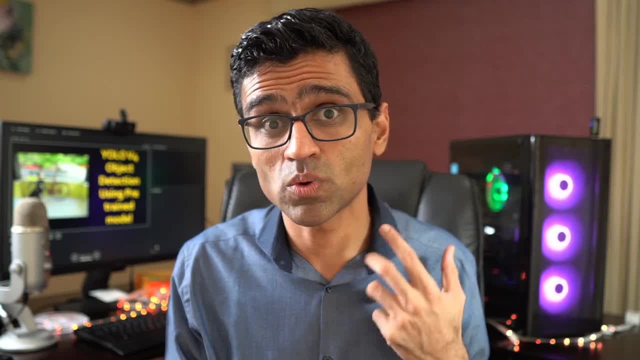 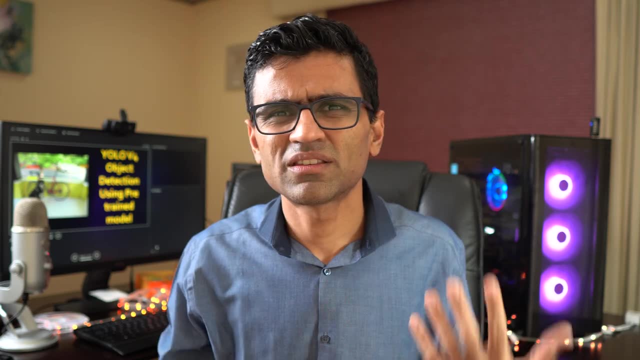 entrepreneurship or freelancing, even options that you have many times people- let's say you're living in india or some asian country- you might be frustrated, or there is traffic, there are no job, the country sucks, but you need to think differently. there are opportunities like if you talk about. 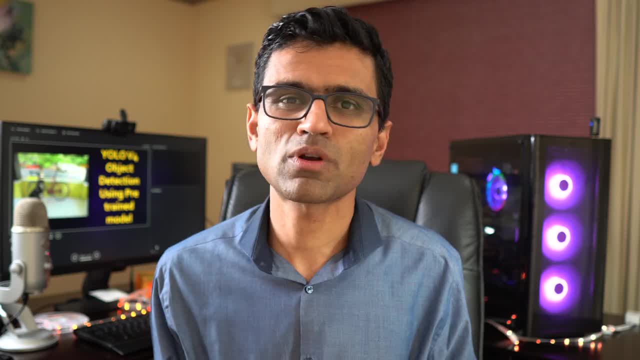 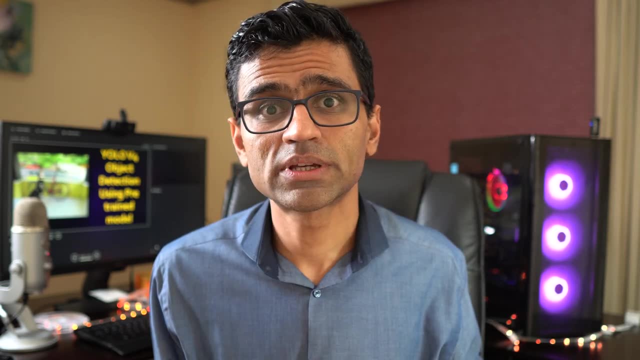 india. there are a hell lot of opportunities. you need to pursue your opportunities. people say: i'm not getting an interview call, i'm not getting a job. well, have patience. you have to do something out of the box. you have to do networking. you have to do a lot of networking. you have to do a lot of. 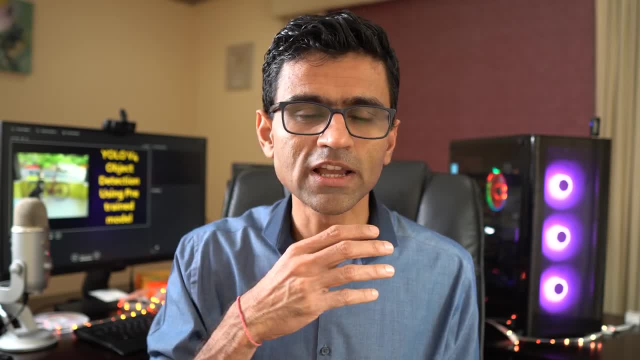 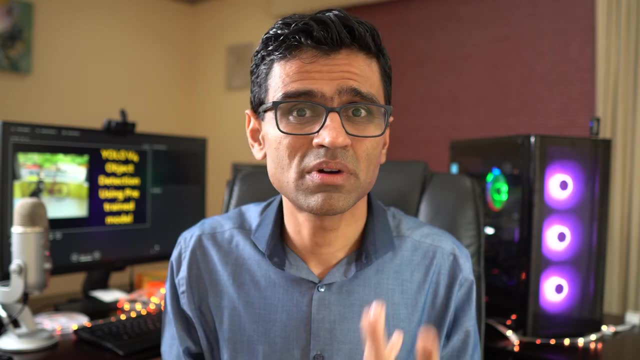 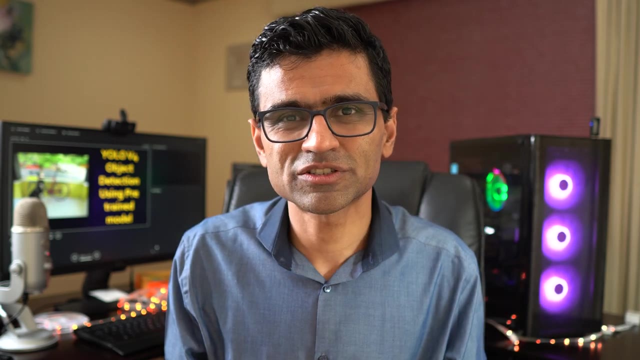 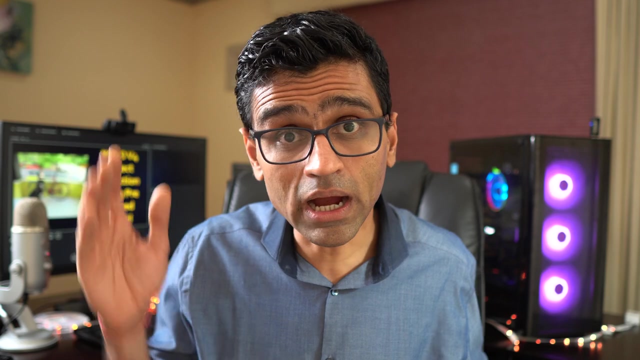 freelancing, open source contribution uh net like networking through linkedin or even writing article in medium or some other blogs. you have to do all of those things. getting the first breakthrough takes time, but after that you can really fly uh, fly high and you can uh achieve a lot of goals. 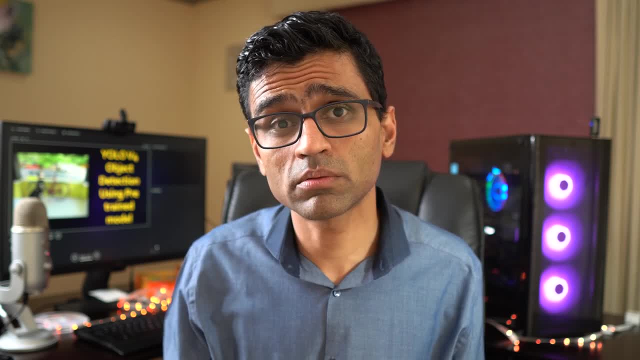 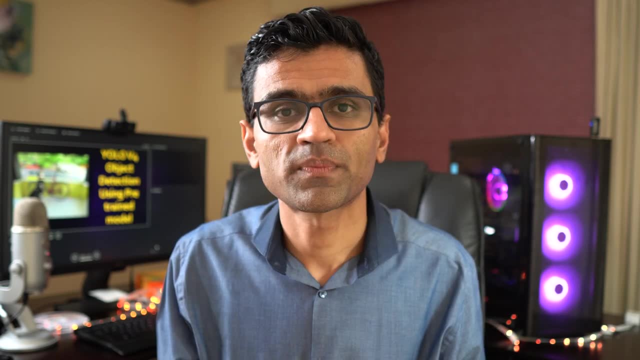 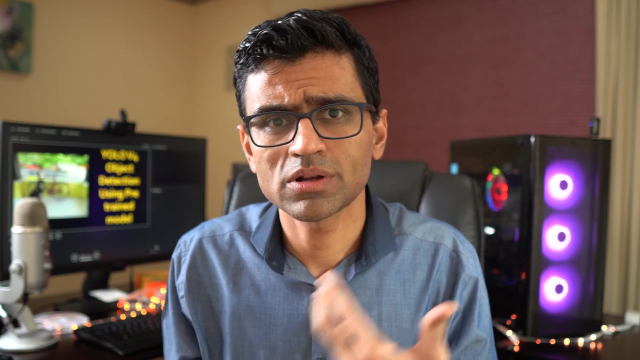 there are many people who end up wanting a lot of money. i mean the, the kind of money that you would not have been expected. you know, as a data analyst, uh in india, you can also have an option of becoming a data scientist. after you become data analyst, you learn the machine learning, predictive modeling skills, statistics, math. you